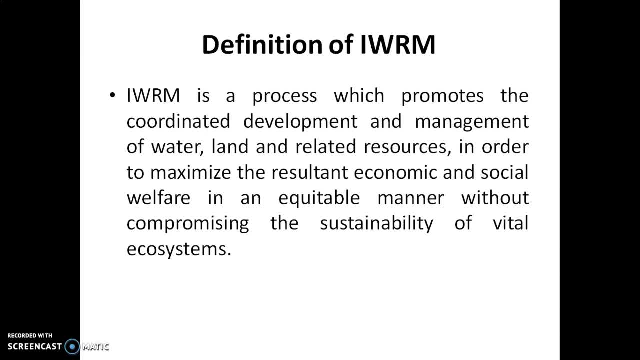 Integrated water source management is a process which promotes the coordinated development and management of water, land and related resources in order to maximize the results of the project. It also promotes the consultant, economic and social welfare in an equitable manner, without compromising the sustainability of vital ecosystem. 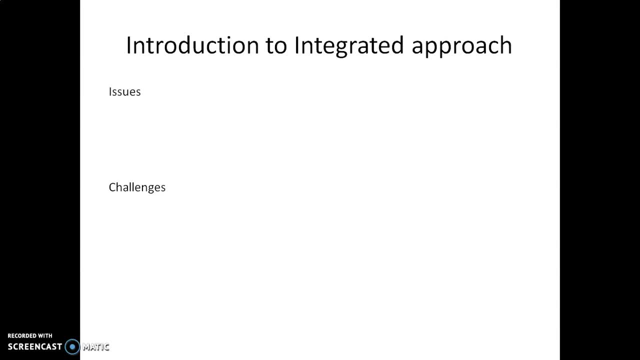 Before introducing the integrated approach of water source management, we need to address 2 important factors: Issues relating to integrated water source management. Issues related to integrated water source management. Issues relating to integrated water resource management. Issues relating to integrated water source management. 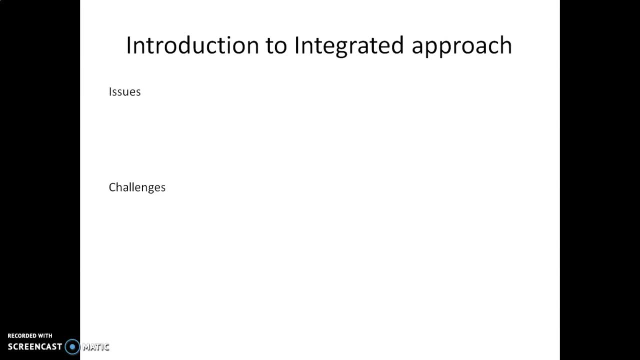 to water source management and challenges will. will take the issues first. the water source: under pressure, only finite quantity of water is available. the population under water pressure- that means increase in population- will demand for more water. impact of pollution: the pollution may be due to natural cause. in most of the cases, the pollution 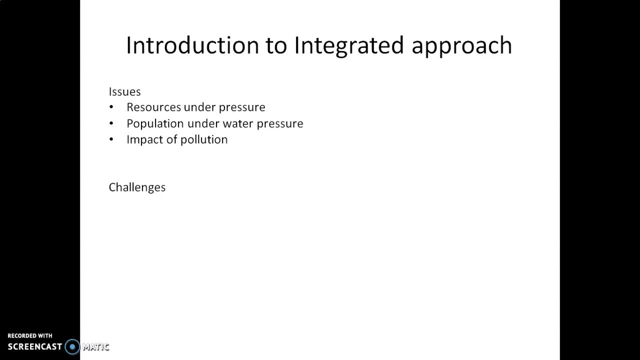 is due to the anthropogenic activity or human activity, water governance crisis, some legislative or administrative related issues in connection with the water management. next we'll discuss about challenges. the first one is the water management crisis. the water management crisis challenge is securing water for people, securing water for food production, protecting vital 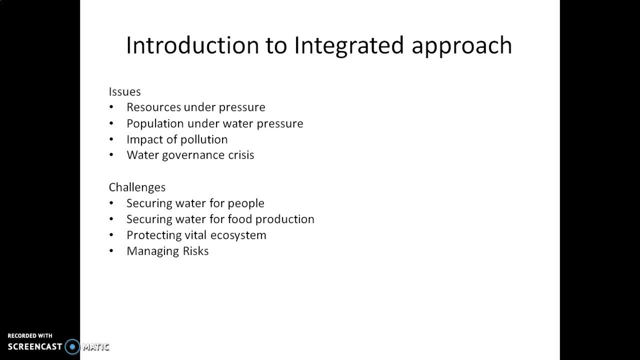 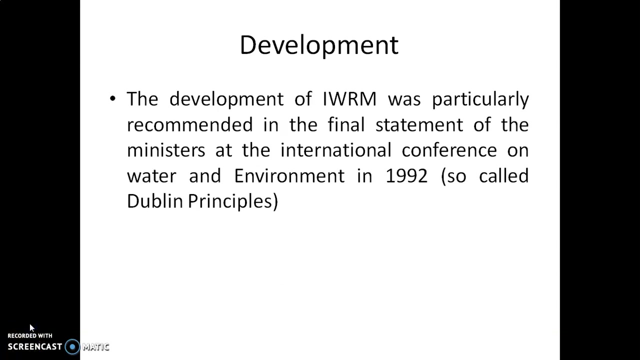 ecosystem, managing risks, developing other job, creating activities, creating popular awareness and understanding, ensuring collaboration across sectors and boundaries. the development of integrated water resource management was particularly recommended in the final statement of the ministers at the international conference on water and environment in 1992, this statement also known as dublin principles. 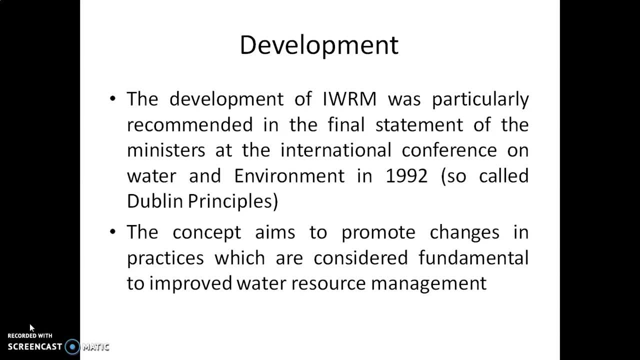 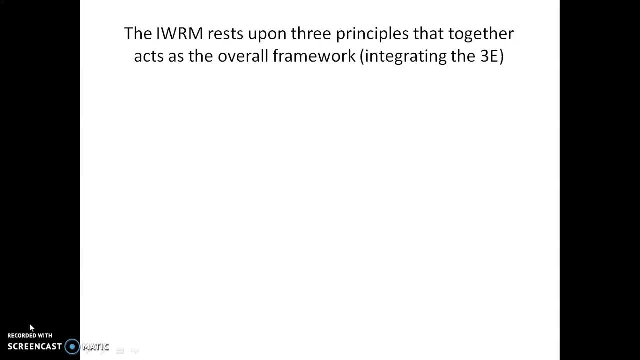 the concept aims to promote changes in practices which are considered fundamental to improve water resource management. the integrated water source management rests upon three principles that together acts as the oral framework. the first one is social equity. ensuring equal access to all users means all people must have access to water of adequate quantity and quality. 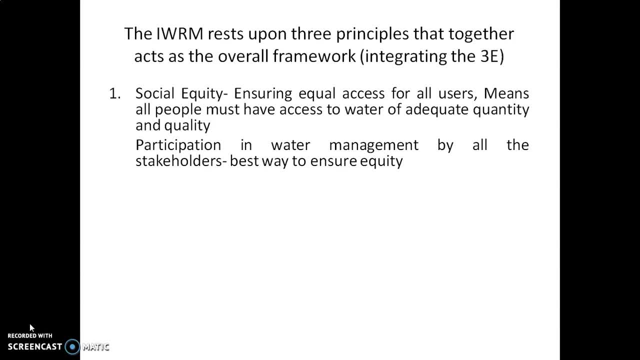 participation in water management by all the stakeholders is the best way to ensure equity. the second point: economic efficiency. efficiency in water use is Forebook integrated waters management. water must be used with maximum possible efficiency by bringing the greatest benefit to the greatest number of juices possibly with. 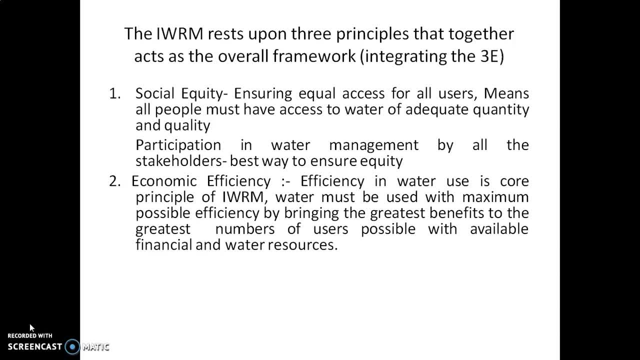 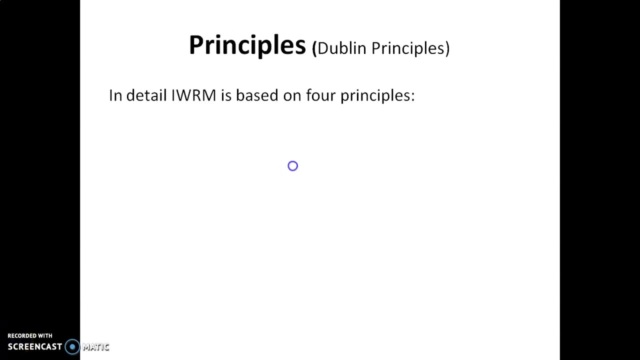 the available financial and water resources that point ecological sustainability. to achieve ecological sustainability, current water use should be managed in such a way that it does not affect the future generation. the principles of integrated water source management. in detail, integrated water source management is based on four principles. these principles also known 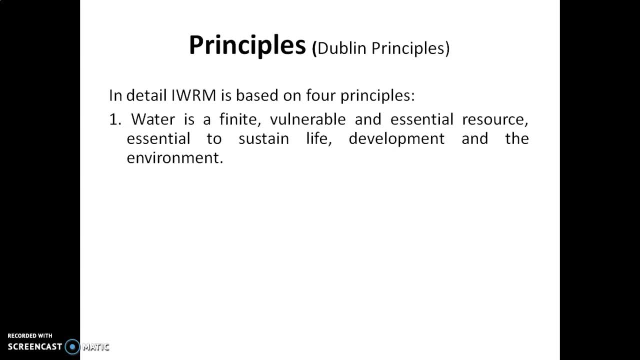 as Dublin principles. the first principle says water is a finite, vulnerable and essential resource, essential to sustain life, development and the environment. the second principle says water resources development and management should be based on a participatory approach, involving users and other resources associated with their conservation of water resources칠387. 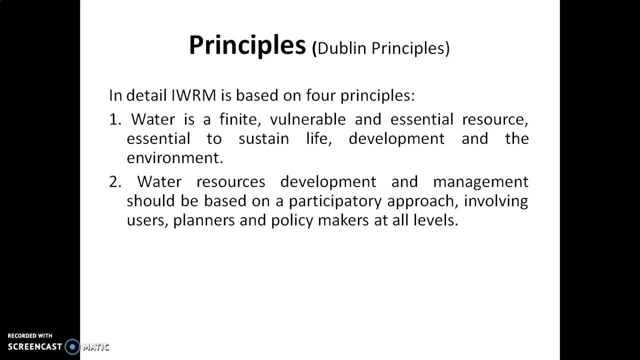 planners and policymakers at all levels. the third principles: very interesting. women play a central role in the provision, management and safeguarding the water. the force principle says water has an economic value. in all its competing uses should be recognized as an economic good. we'll discuss the about. 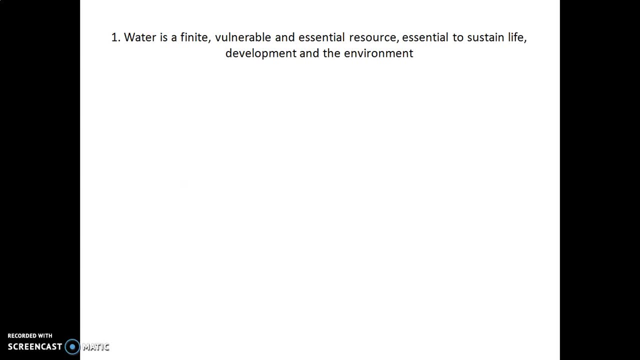 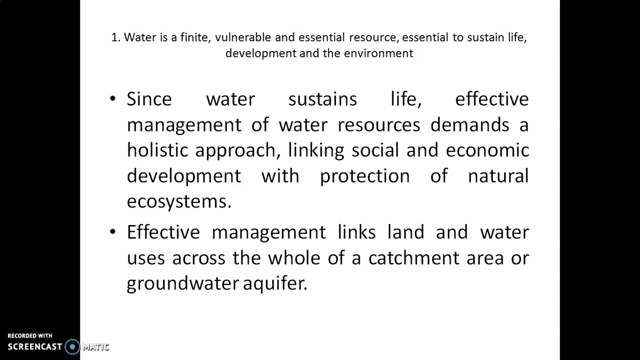 the first principle. that's about water is a finite, vulnerable and essential resources essential to the sustained life, development and the environment. since water sustains life, effective management of water resources demands a holistic approach linking social and economic development with the protection of natural ecosystem. effective management links land and water. 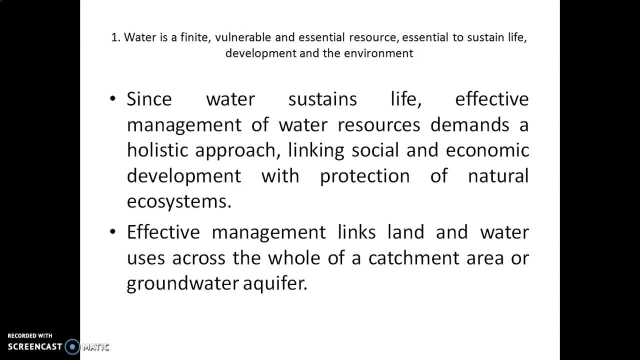 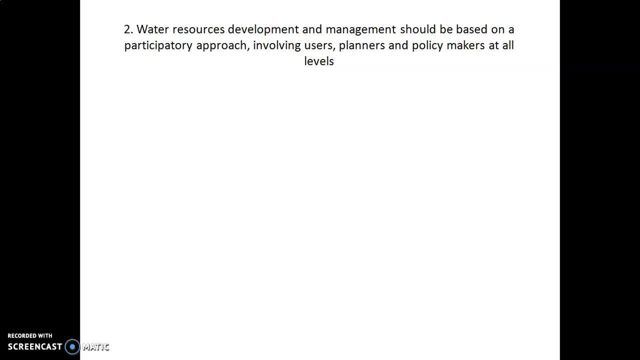 uses across the whole of a catchment area or groundwater aquifers. the second principle says what our resource development and management should be based on: a participatory approach involving users, planners and policymakers at all levels. we'll have discussion on that. the participatory approach involves raising awareness of potential activities and equation also. 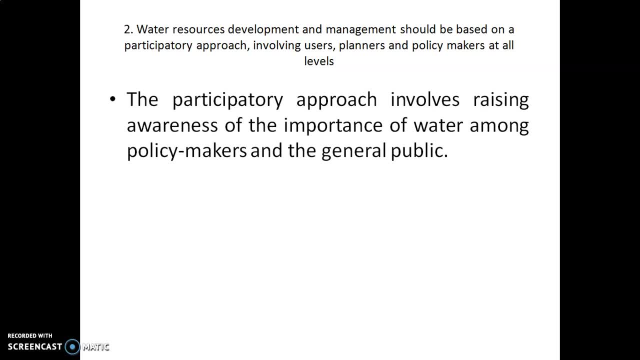 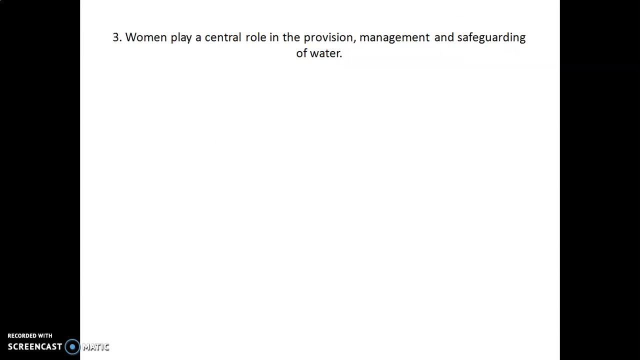 needs a lot of envelope management in foreign lands, such as on droughts. from the rising awareness of the importance of water among policy makers and the general public, It means that decisions are taken at the lowest appropriate level, with full public consultation and involvement of users in the planning and implementation of water projects. 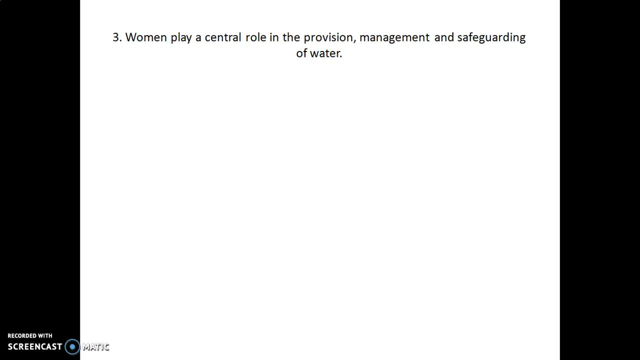 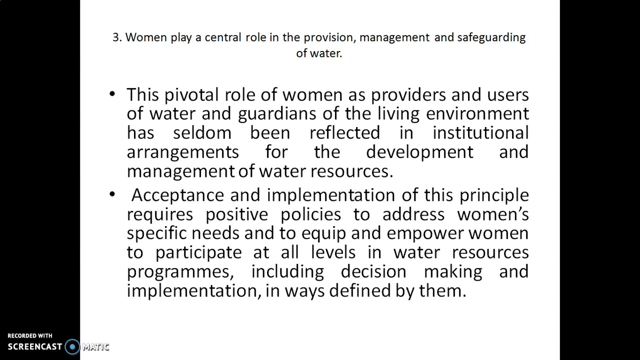 Third principle says women play a central role in the provision, management and safeguarding of water. This pivotal role of women as provider and users of water is very important. The importance of water and guardians of the living environment has seldom been reflected in institutional arrangements for the development and management of water resources. 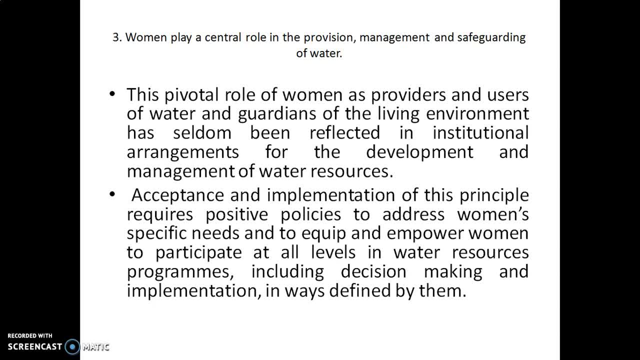 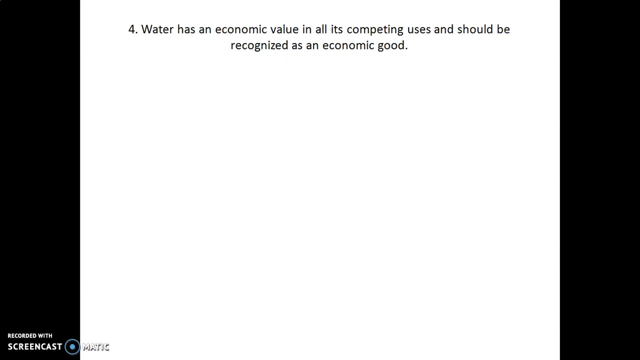 Acceptance and implementation of this principle requires positive policies to address women's specific needs And to equip and empower women to participate at all levels in water resources programs, including decision-making and implementation in ways defined by them. Fourth principle says water is an economic value in all its competing uses. 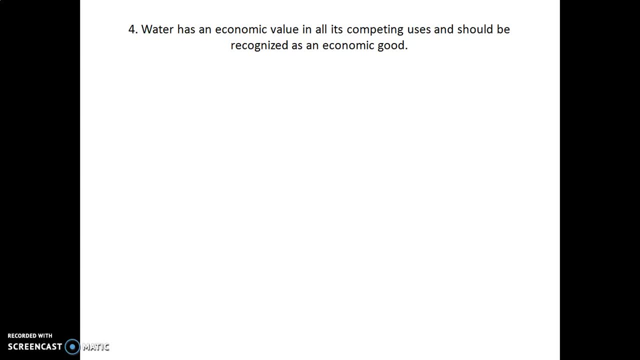 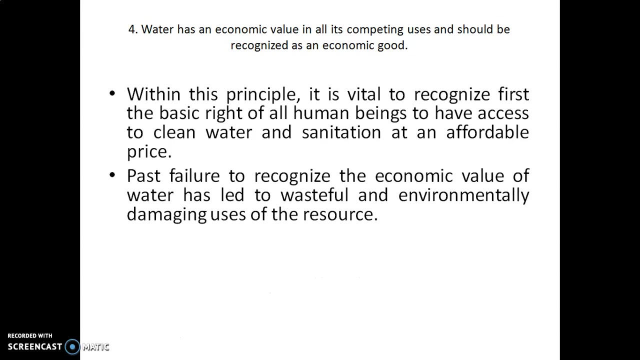 And should be recognized as an economic good. Within this principle, it is vital to recognize first and basic right of all human beings to have access to clean water and sanitation at an affordable price. They get it. There is no reason they don't get it. 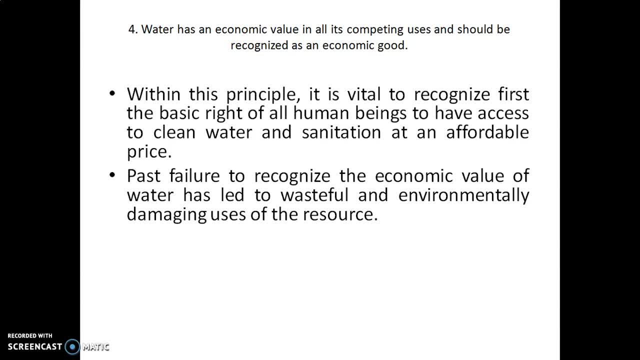 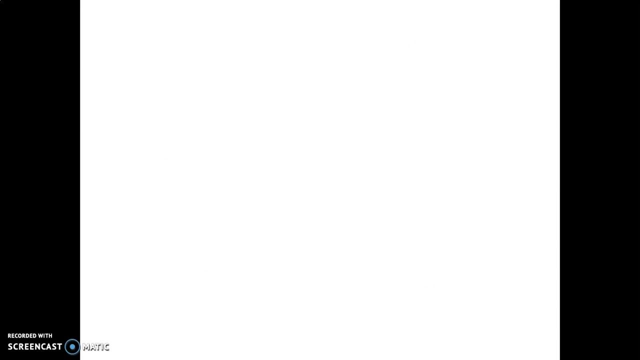 Why, Why, Why? economic value of water has led to wasteful and environmentally damaging uses of the resource. managing water as an economic good is an important way to achieving efficient and equitable use and of encouraging conservation, of conservation and protection of water sources. thank you.